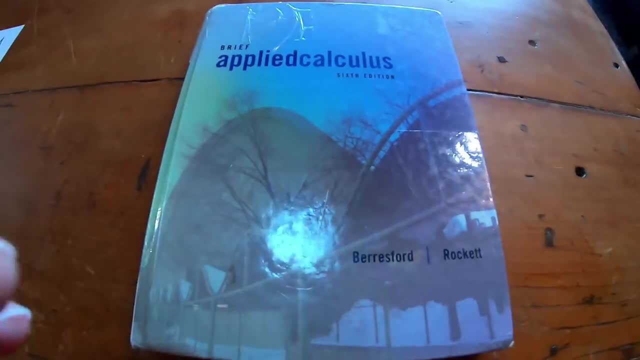 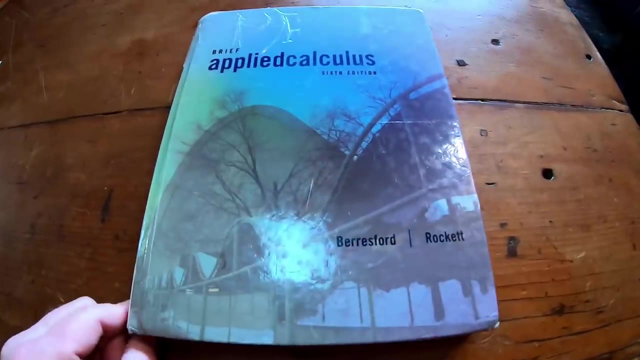 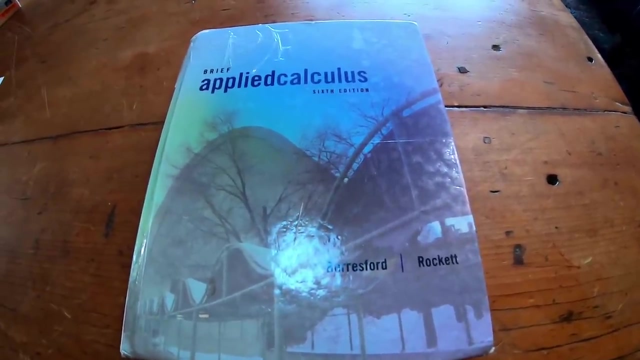 and it's by Beersford and Rocket. And the reason that this is a shortcut way is that this book requires zero trigonometry. Okay, with a book like this, you can learn calculus without knowing any trig. Now you do need some algebra, but only like basic algebra, Right, you need to be able to like. 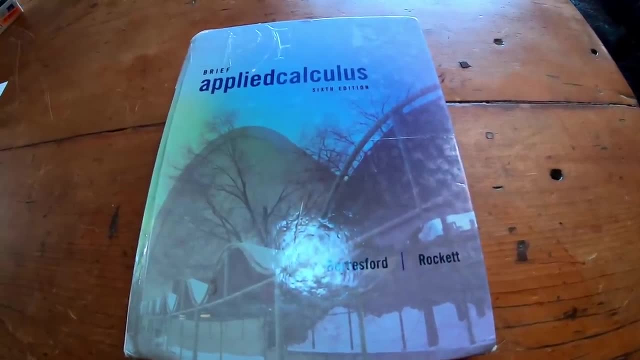 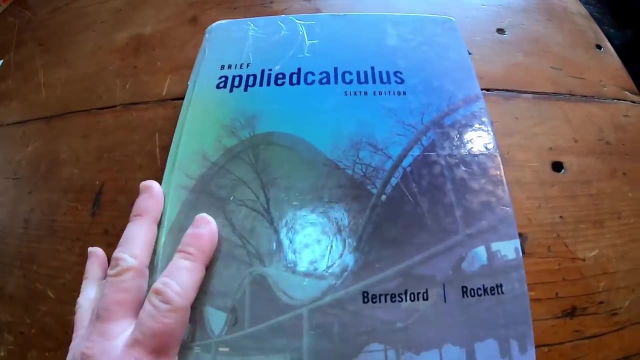 distribute things and just do basic operations with exponents and stuff like that. So this is it. This is an awesome book and you can get a used copy on the internet if you do some research- for just a few dollars. I'll leave a link in the description. but this is a nice way to jump into it. So if you want, 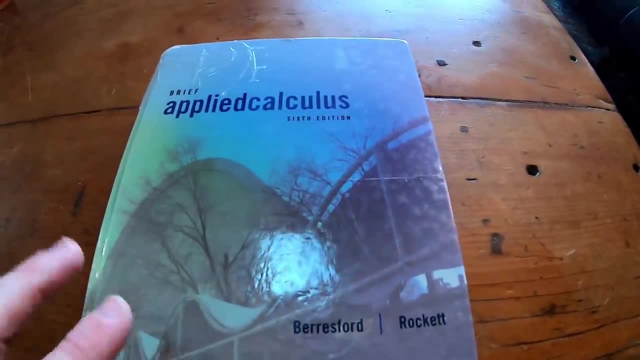 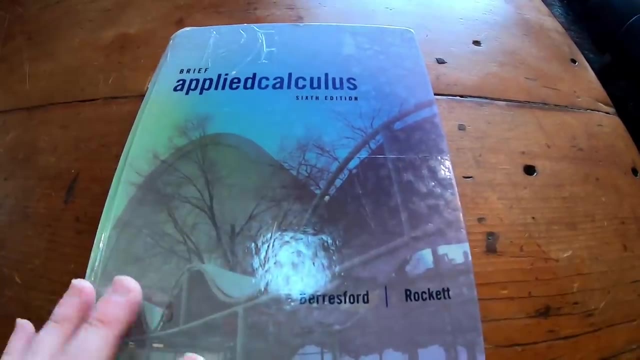 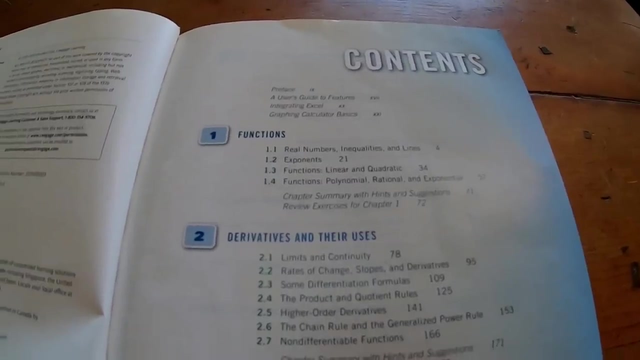 to get into calculus and you want to skip the trig, this is a way to do it. Now, eventually you'll have to go back and like learn trig if you want to get into some higher level stuff. But this book, this book covers a lot. Let me just quickly show you some of the topics in this book. So this book has 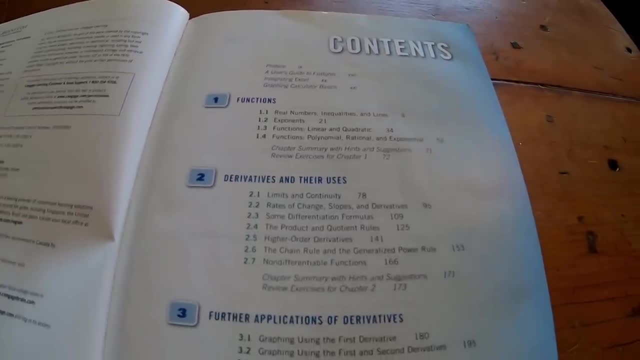 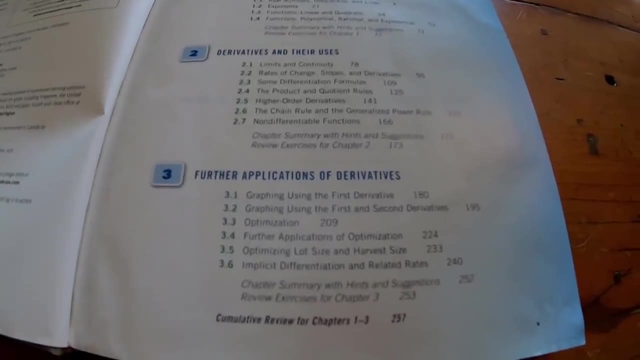 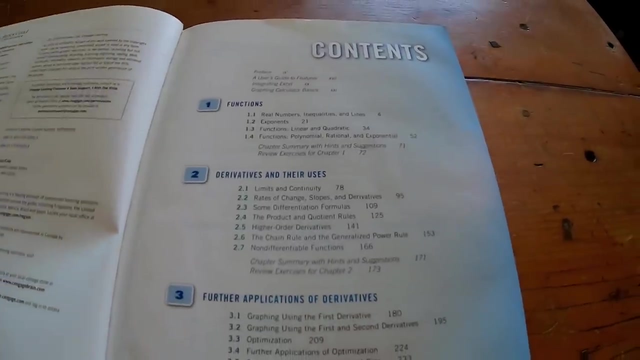 parts of calculus. It doesn't cover everything that a regular calculus book would, but it covers the basic stuff. talks about derivatives, some applications of derivatives which you wouldn't find actually in a regular calculus book. that has like business applications, stuff like that Typically this book is used for like a course called business calculus or concepts of calculus. 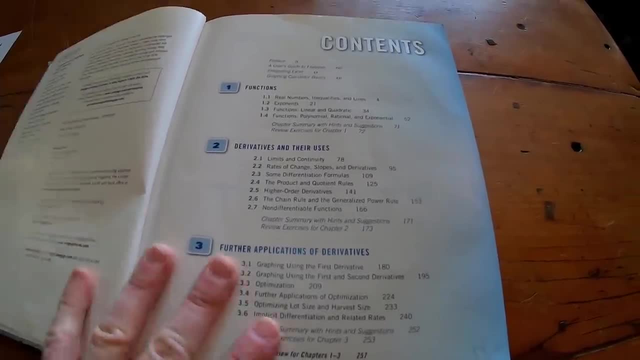 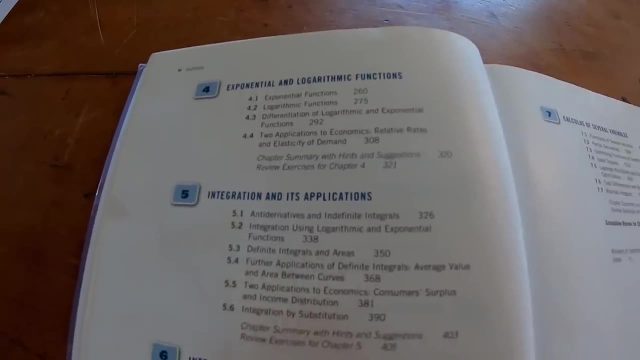 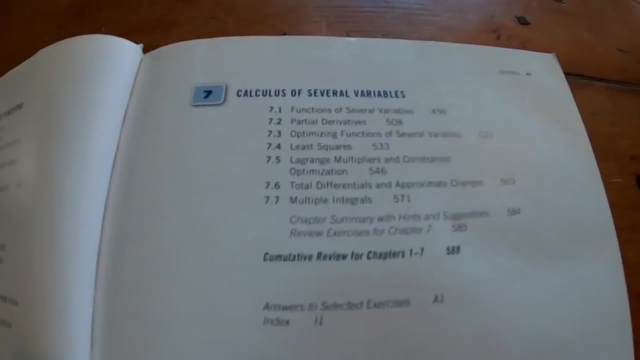 non science majors, non math majors, would use a book like this. So it's written at a very, very introductory level. Let me turn the page. It talks about the exponential and logarithmic functions, then talks about some integration techniques and over here it talks about calculus of several variables. So it actually has selected. 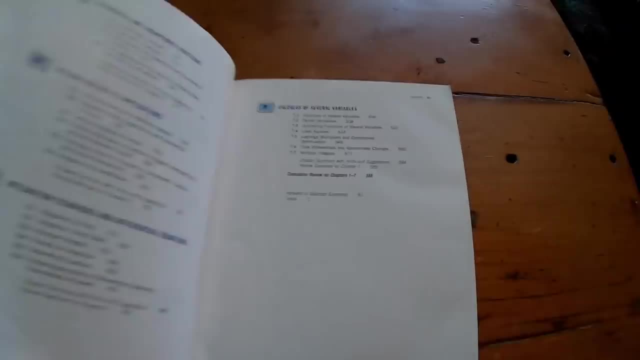 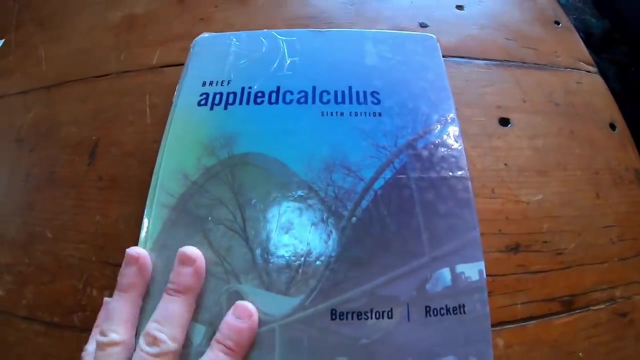 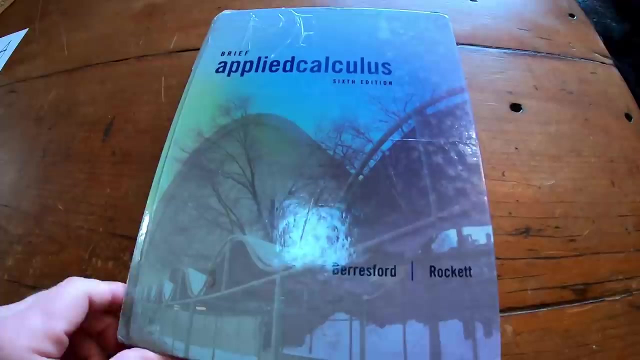 topics from calc one, calc two and calc three. So this book actually has topics again from all three calculus courses- one, two and three- and it avoids trig. So it's a good way, it's a really good way to jump into it. So if you don't want to like get bogged down with all that algebra and trig, you 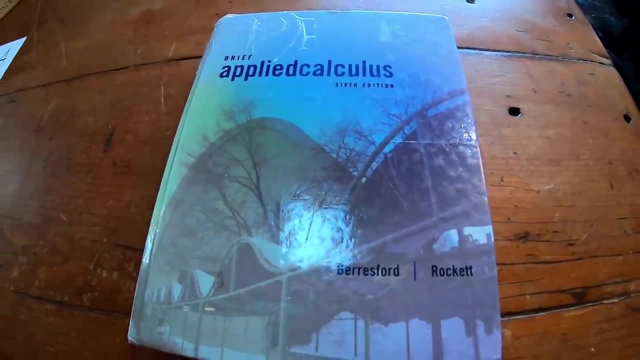 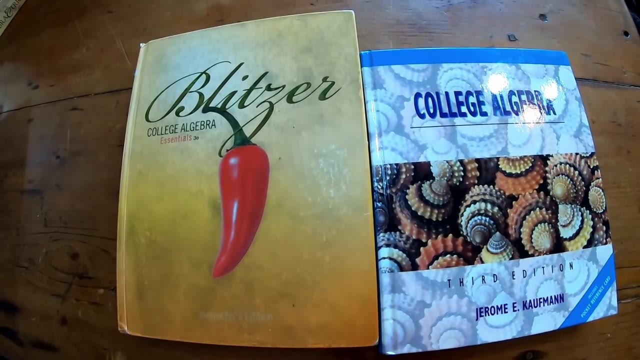 can just jump into this A little bit and actually just start learning calculus right away. So if you want to learn calculus the traditional way and you want to work your way up to trig, or if you need in like an algebra refresher, these are really two really good choices. This is college algebra by 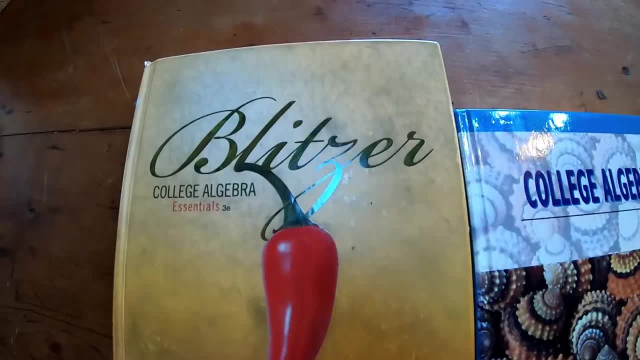 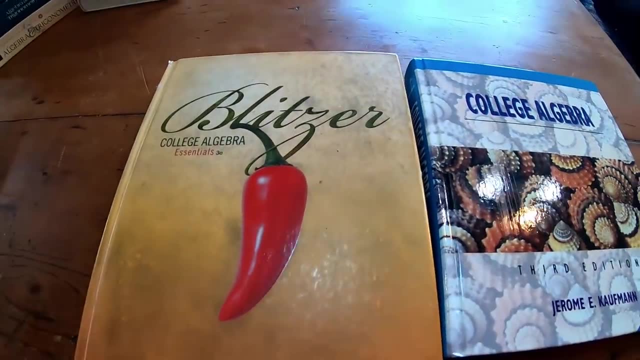 Blitzer. It's a really, really good book for college. algebra covers more than what you need, And this is the one by Kauffman, and this one's a little bit easier to read, And both of these can be purchased for just a few dollars on the Internet. So if you need a refresher, 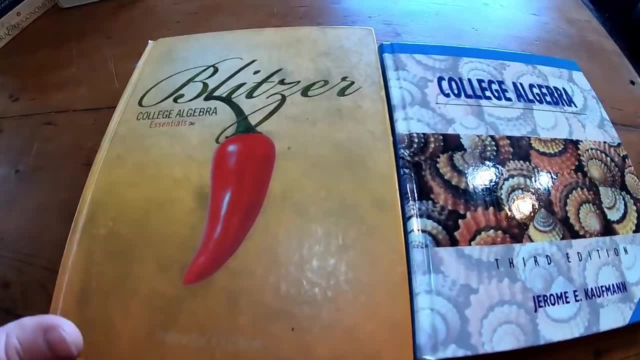 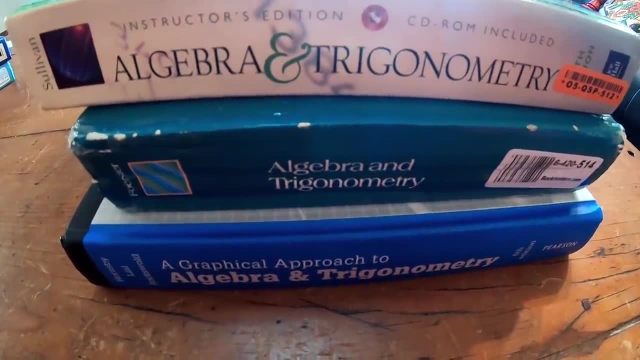 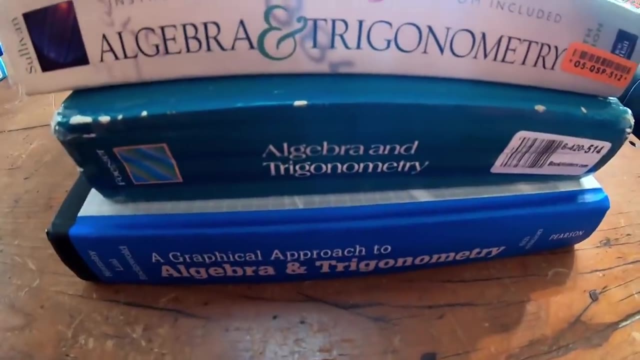 These are pretty good books, but again, this video is about calculus, So let's keep going. So here we have three books on algebra and trigonometry, So these books cover both algebra and trig. These are usually used in colleges and universities to teach courses called pre calculus and also courses called trigonometry. 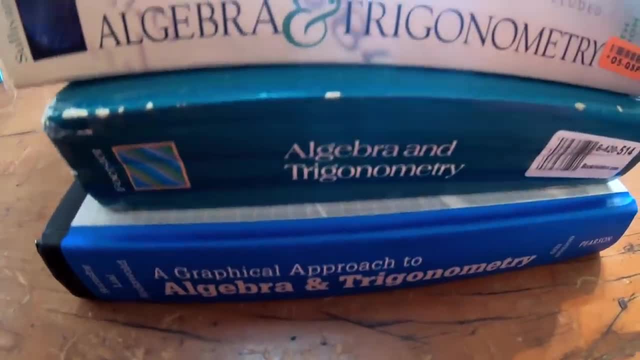 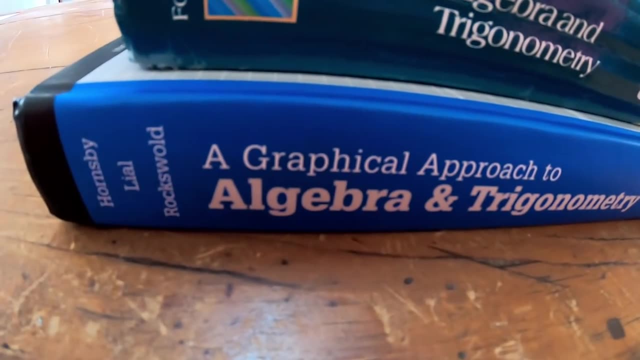 Now the algebra problems in these books are harder than the algebra problems in the books that I showed you before these, So in theory you can just get one of these and that should be enough. I like this one, The one by Hornsby, Lyle and Roxwold, A Graphical Approach to Algebra and Trigonometry. 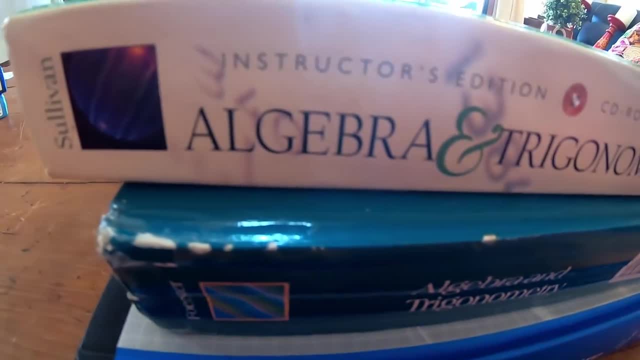 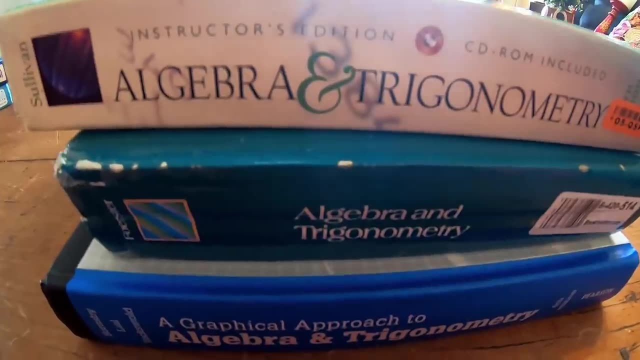 The one by Forrester is pretty good and the one by Sullivan is a classic: Algebra and Trig by Sullivan. So all three of these are pretty good books to refresh your trig or learn trig and refresh your algebra. Okay, let's go into the calculus. 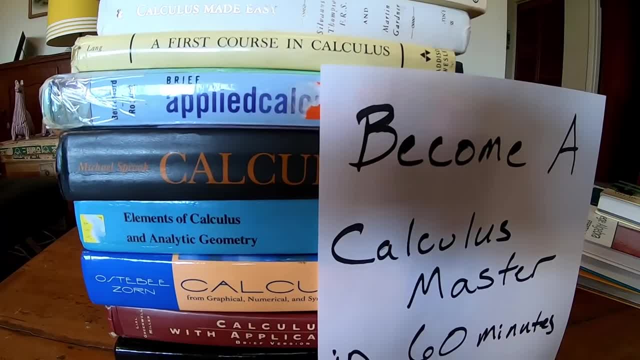 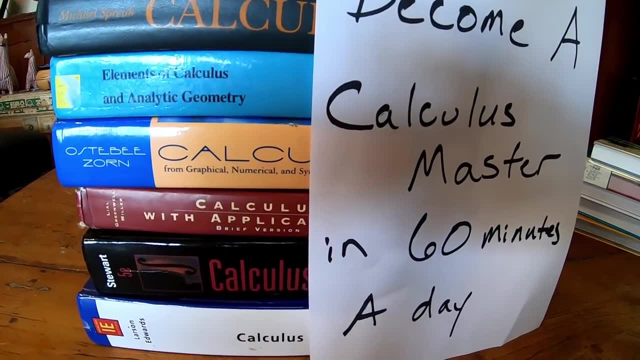 So here I've picked some of my calculus books, And so what you want to do with these books is you want to spend 60 minutes a day, at least 60 minutes of focused study time. So that means you are doing nothing else but working on calculus. 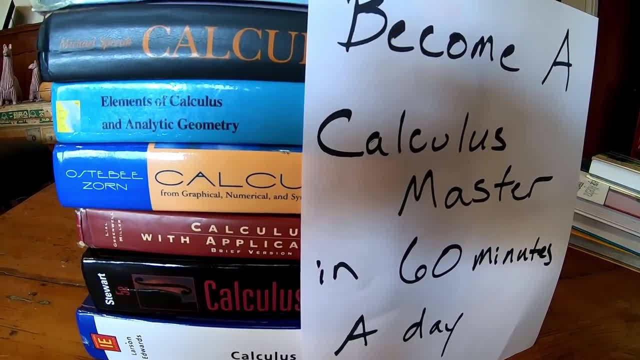 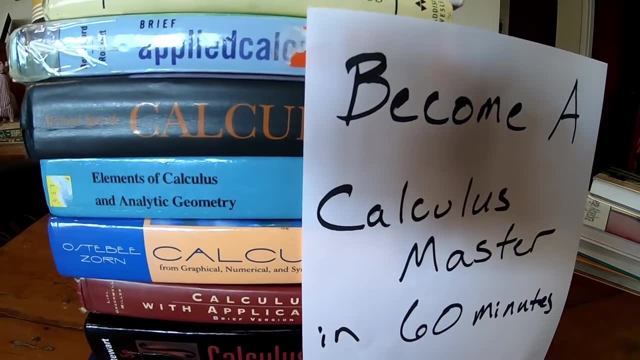 So you're either reading or working out problems, but you want to time it and you want to try to spend at least 60 minutes a day. You can spend less and, honestly, any time you spend doing math is better than no time. 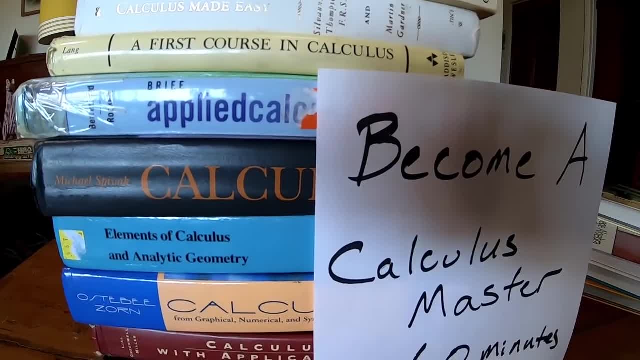 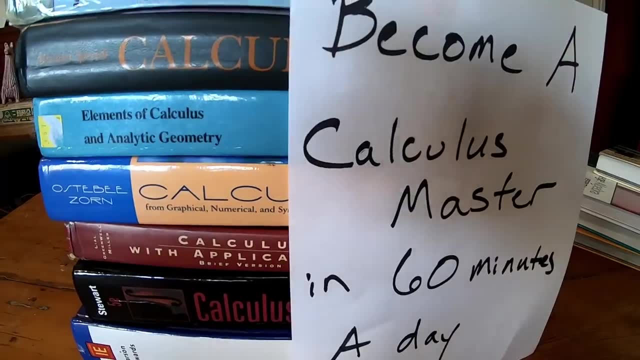 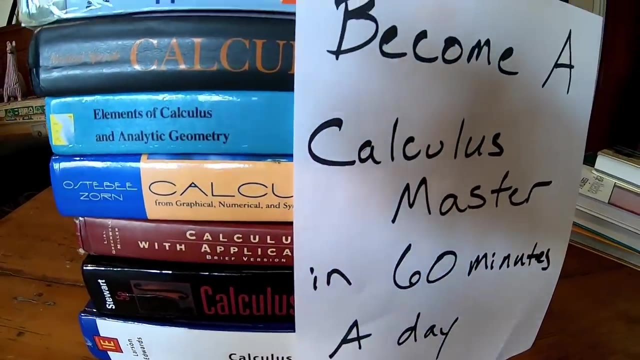 And on those days that you don't want to do it, if you kind of just sit, Sit down and just say: hey, I'm going to spend one hour of my life learning calculus, It will help you so much. You will not believe how much better you will get if you just spend 60 minutes a day. 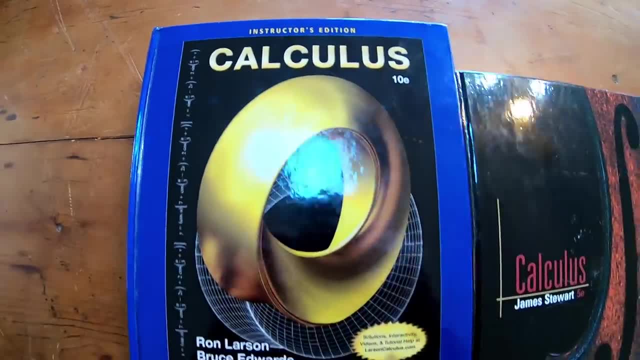 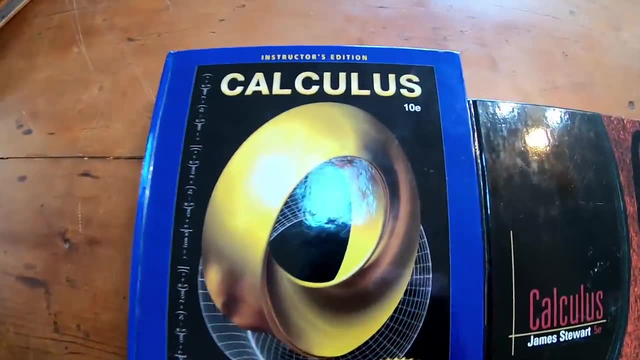 So let me show you a good way to start with this. So both of these books are pretty equal. This is the one by Larson, Calculus by Larson and Edwards, And it's used at most colleges and universities, along with the one by Stewart. 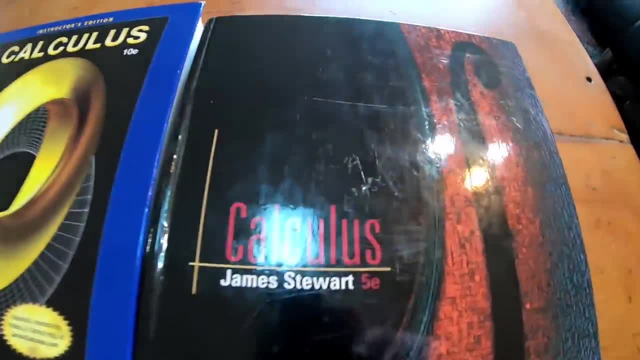 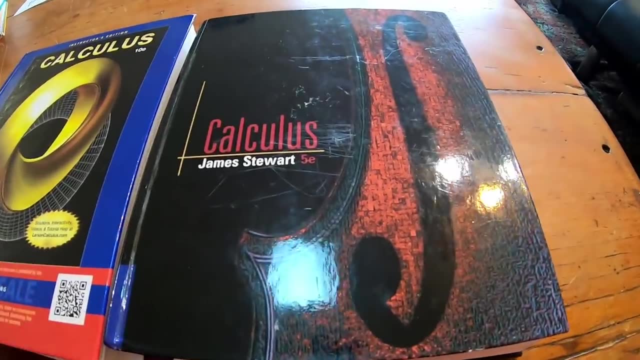 So These are probably the two most popular. The one by Stewart, this one here, Calculus by James Stewart, is probably the most popular calculus book in the entire world. Now, these books aren't perfect. They're calculus books, so it's better to have more than one. 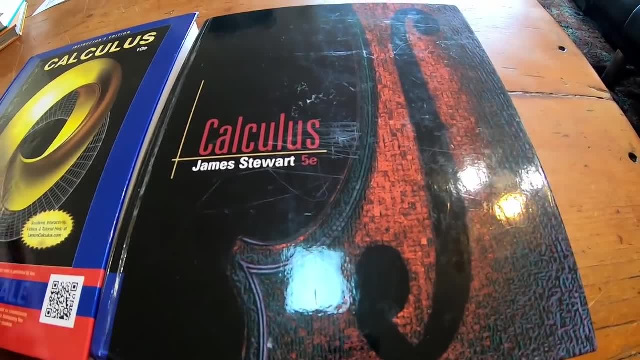 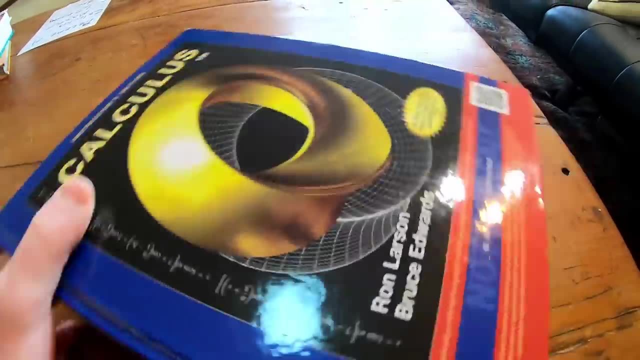 And so, again, what you want to do is you want to just spend at least an hour a day reading or working through problems. And these books shine in one regard: Mainly these books, These two books are awesome for Problems because they have so many problems. 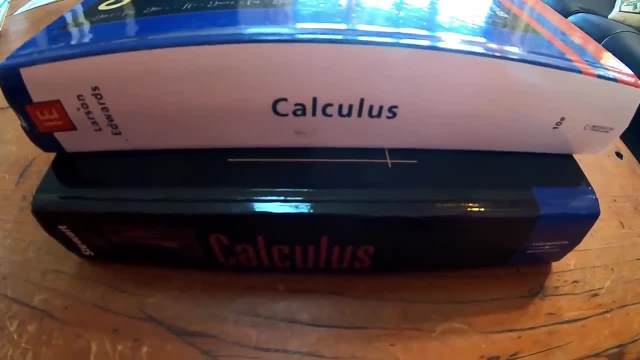 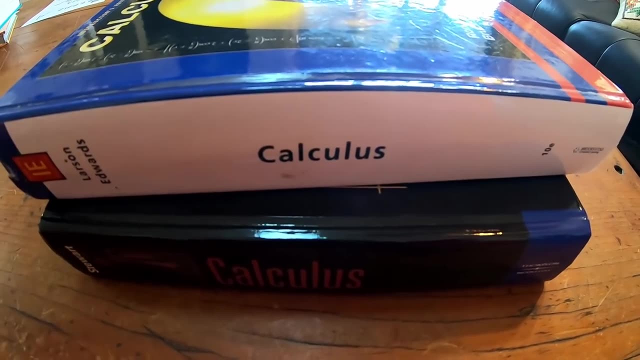 They also have lots of pictures that explain the concepts, which a lot of the other books don't have. So that makes it a plus. And again, you can get these for just a few dollars used. If you go on the Internet and you look for used copies, you can probably find one pretty inexpensively. 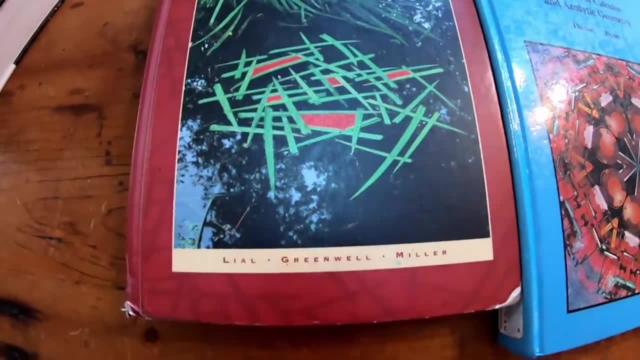 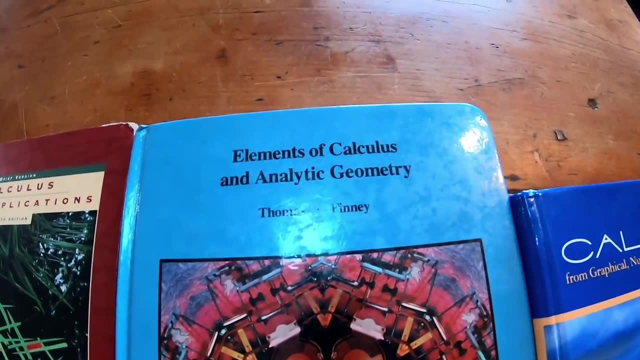 Here's a couple more. This is the one by Lyle Greenwell, and Mailers is a pretty good calculus book. This is actually one of my favorites, And I actually have not done a review on this one And I will. This is the one by Thomas and Finney. 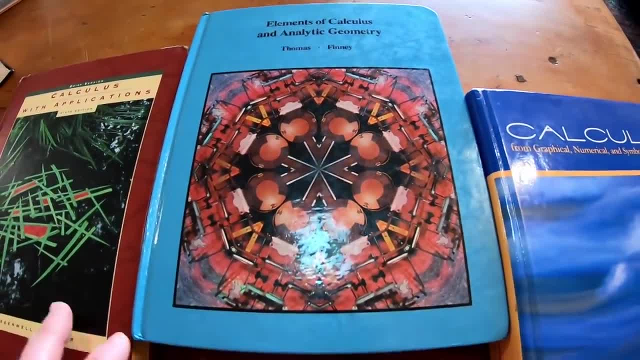 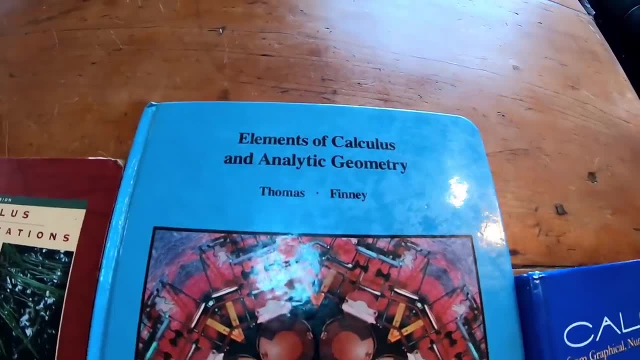 I've actually been reading this recently. I love this book. I have so many good things to say about it. I would highly recommend this one: Elements of Calculus and Analytic Geometry by Thomas and Finney. I love this book, And here's one you've probably never heard of. 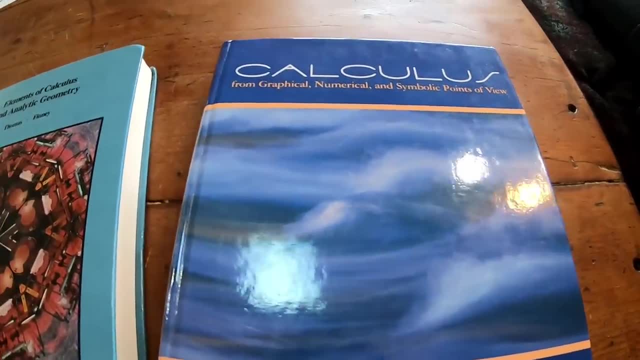 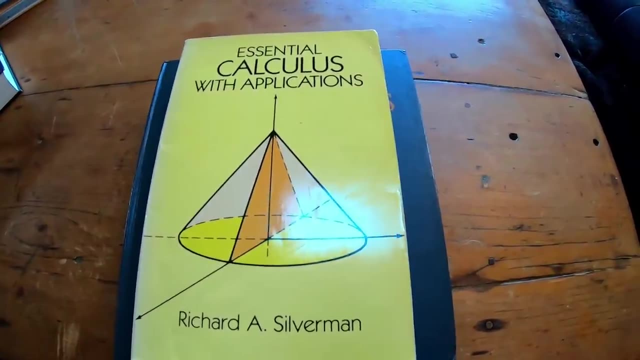 This is the one by Ostebi and Zorn, So any of these is good, But I still recommend the previous two because of their source of problem. Here's another one. If you're on a budget, you can Probably definitely get this cheap. 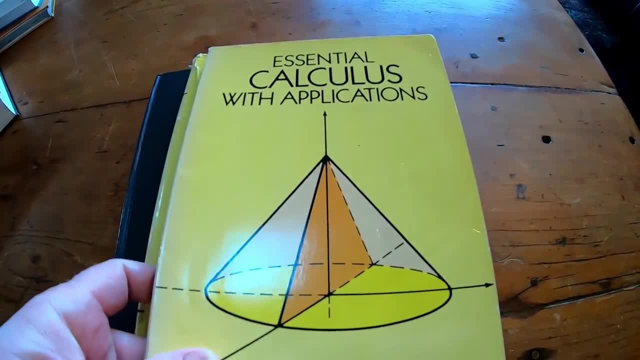 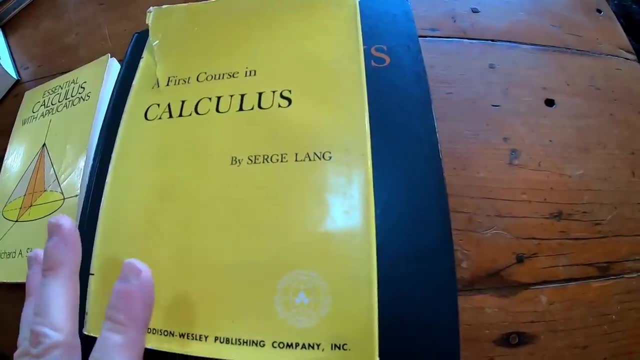 This is the one by Silverman. It's a Dover book, So it's quite an expensive. Let's keep going. Here we have the famous A First Course in Calculus by Serge Lang. This one's really good too, But you'll probably find it lacking compared to some of the other ones I showed you. 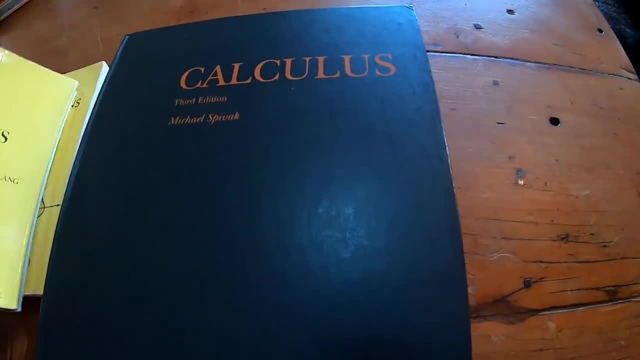 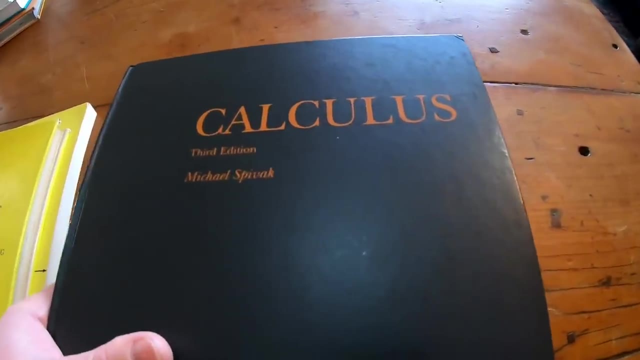 But a used copy is not so expensive. If you are willing to spend more money, this one's going to cost a little bit more. It's not going to be like $10.. This is Calculus by Michael Spivak, And the thing with this one: 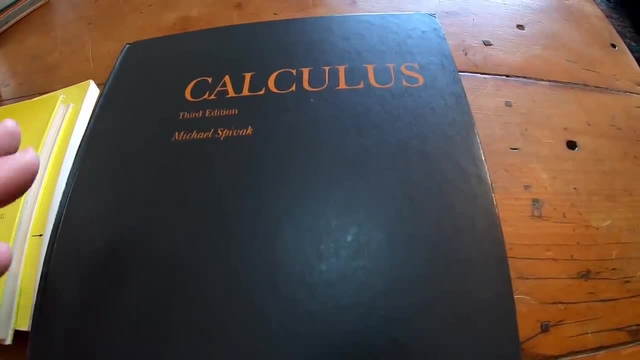 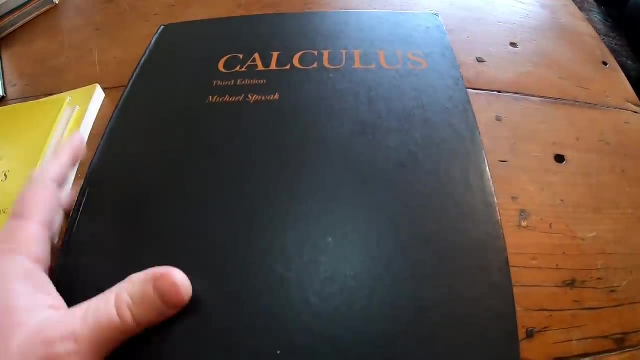 Is. it's a great book. It reads better than all the other ones, But you might have a harder time understanding it. But if you really want to become a calculus master, I kind of feel like this is one of those must-have books. 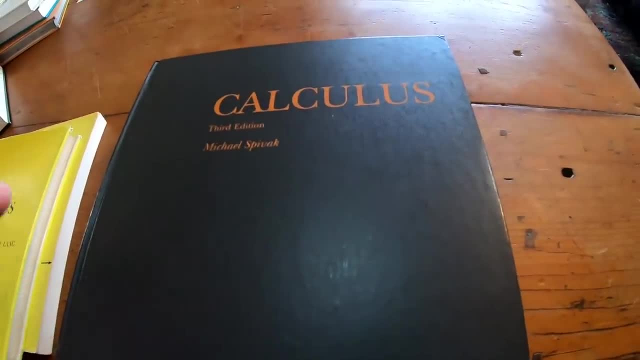 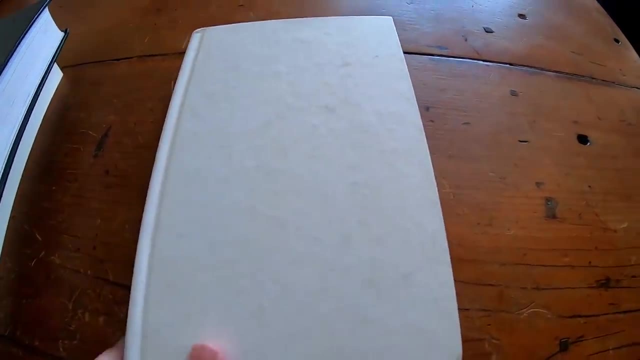 You know, you buy it and you just keep it for the rest of your life. you know, And then you read it from time to time. At the very end, we have this little white book. This is a book that you would read when you go to bed. 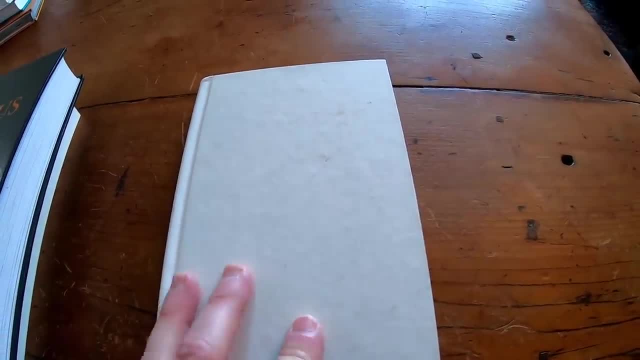 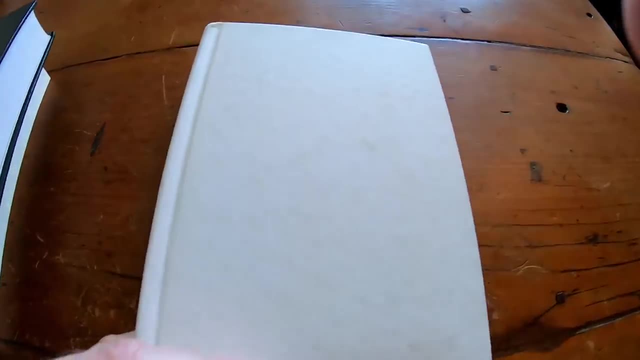 So you read this as part of your 60 minutes, or in addition to This is Calculus Made Easy By Thompson. This is an amazing book And it's very, very good And it's a good complement to the other calculus books. 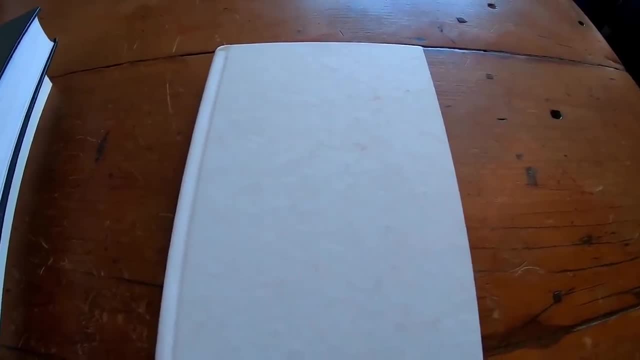 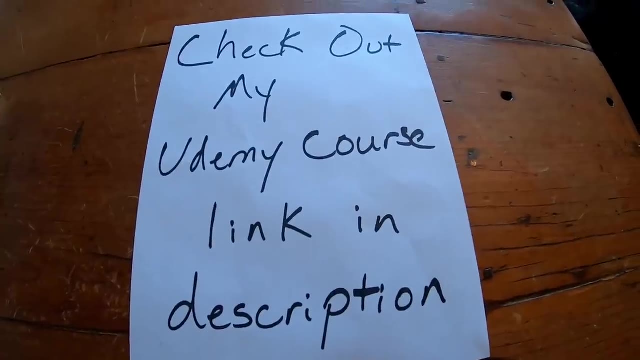 So what else can you do besides read calculus books? Well, there's videos to talk about that. So obviously this is a YouTube channel, So I have, like, lots of math videos. You can watch the videos also, And that can also count for your 60 minutes a day. 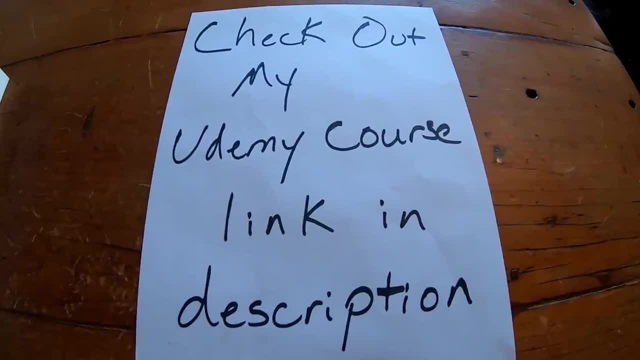 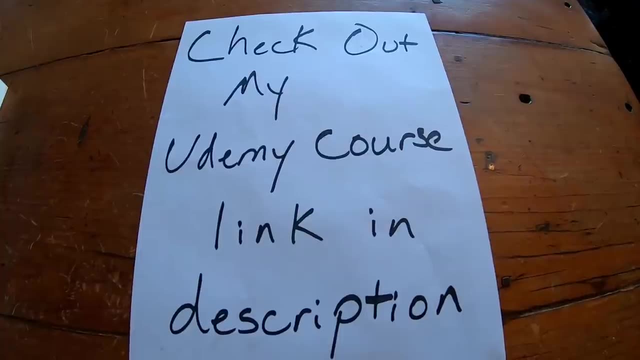 And I also have Calculus 1 lectures on my channel, So I have a playlist on my main page And actually I have a playlist on my main page And it actually has full lectures on Calc 1 that you can watch. And I do have courses on Calc 1,, Calc 2, Calc 3 on Udemy. 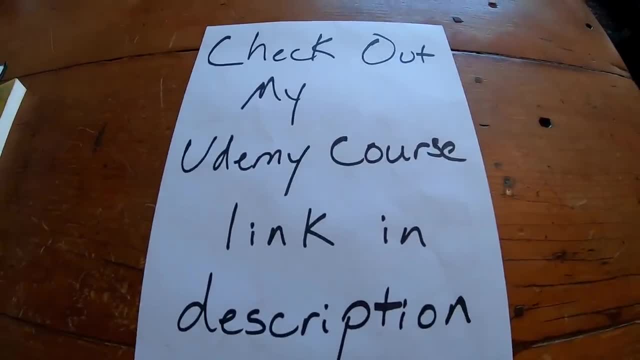 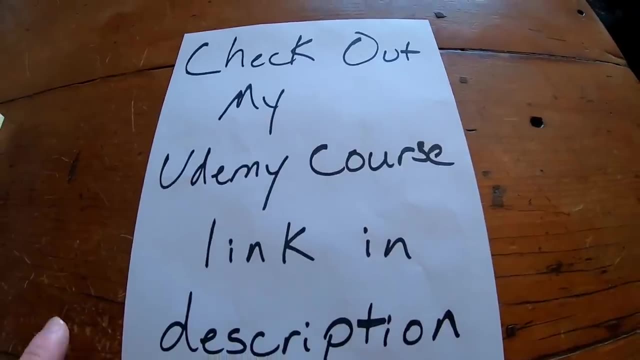 And I usually don't pump these ever. I don't think I've ever mentioned them in a video. There's always a link in my descriptions, But I don't know, It just doesn't feel right. But they're there And they're not that expensive. 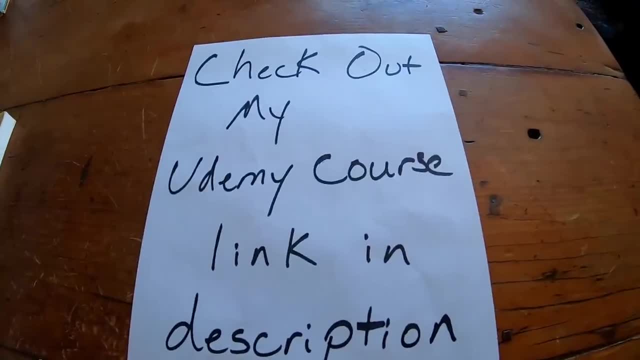 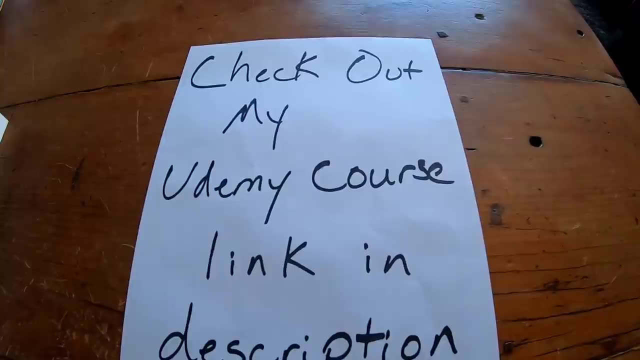 And I have them for Calc 1,, Calc 2,, Calc 3.. And also for college algebra. And in my opinion- this is just my opinion- I think my college algebra course and my Calc 1 course are better Than the other ones. 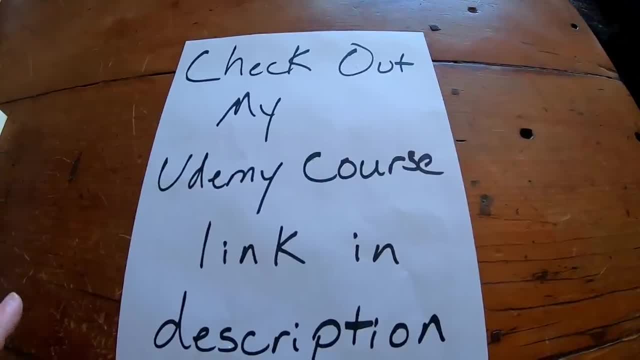 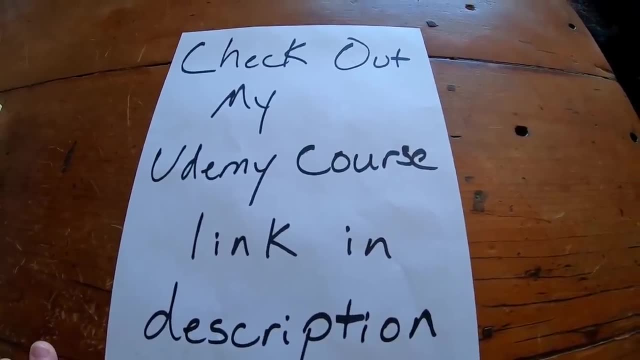 Because they actually have assignments. My college algebra course and my Calc 1 course actually have assignments And I just feel they're more complete because of the assignments. So yeah, That's it. So to become a calculus master, all you have to do is spend 60 minutes a day. 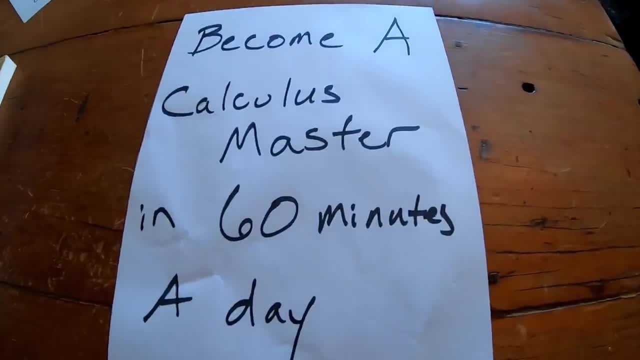 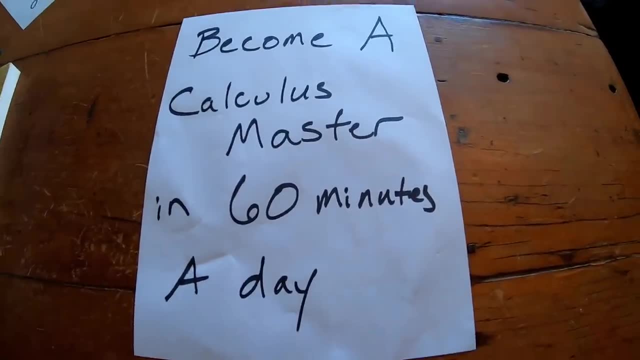 So all you do is take 60 minutes of focused study time. So what I mean by that is you have no distractions. You are just purely focused in the moment, Like you want to live in the moment, like a dog. You ever seen a dog laying in the grass? 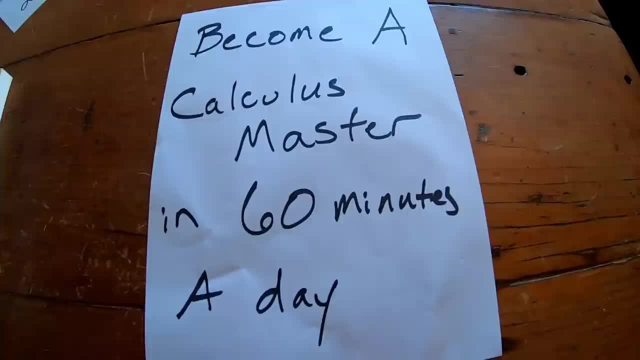 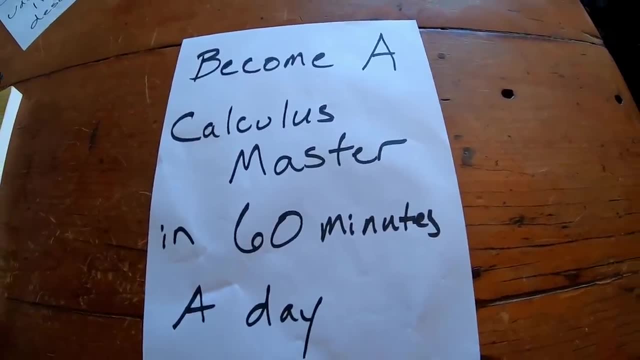 It just lays there and rolls and enjoys the sun. It's the same thing, But you want to roll around and enjoy the calculus. That's why I like books. Instead of smelling the grass, you smell the books. So I hope this video has helped you. 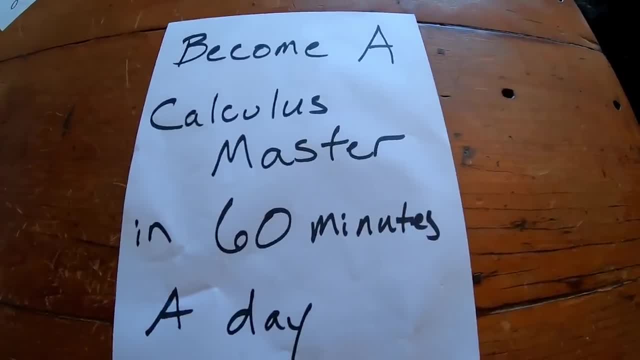 And try to do it. Try to become a calculus master. Let me know what you think in the comments below. Good luck. 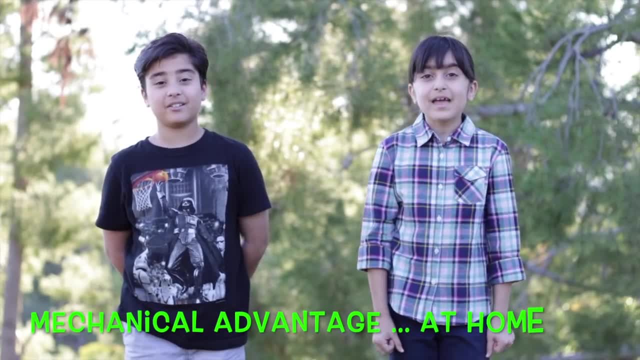 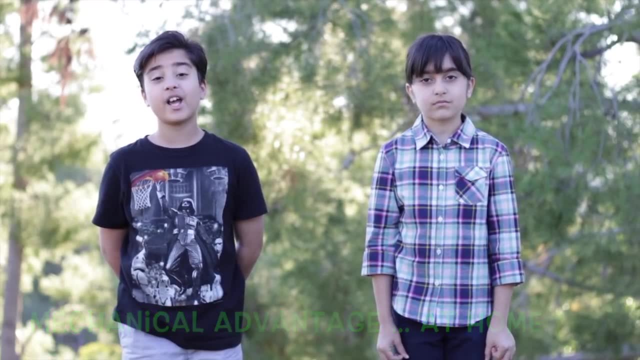 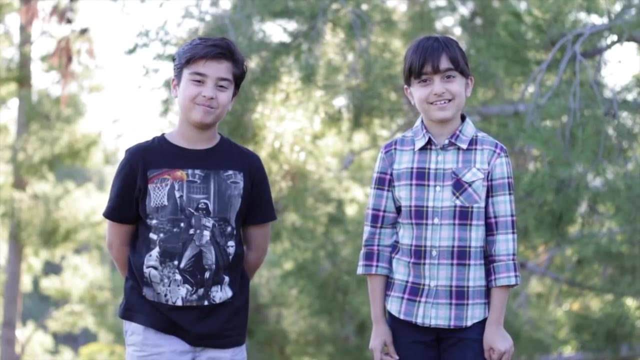 Hello. I'm Sophie And I'm Alex, And we are the Science Kids. Today, we'll talk about a very important phenomenon that is found everywhere and has made such a difference in the history of science: Mechanical advantage. Mechanical advantage is what allows you to carry your 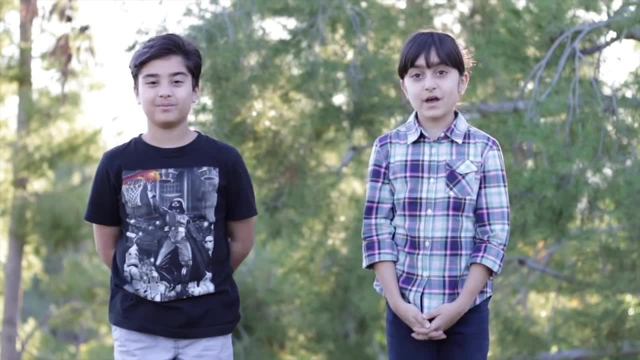 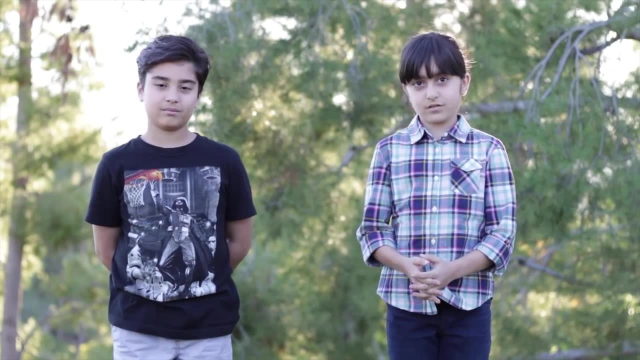 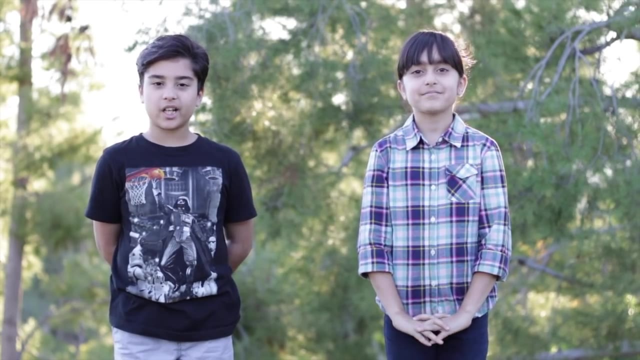 heavy grocery bags without complaining at all. They also allow you to carry bricks without hurting your fingers or dropping them on your toes, Though some basic mechanical devices we use on a daily basis are levers and pulleys. The Statue of Liberty was brought to the United States. 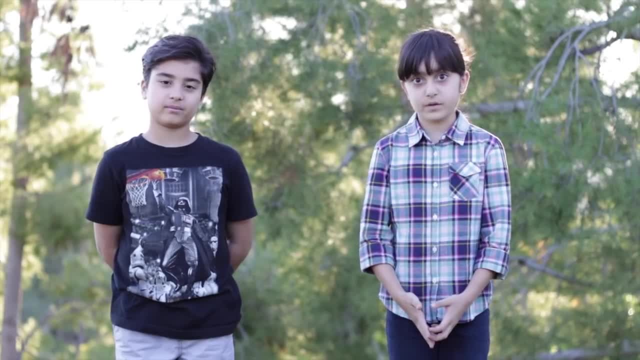 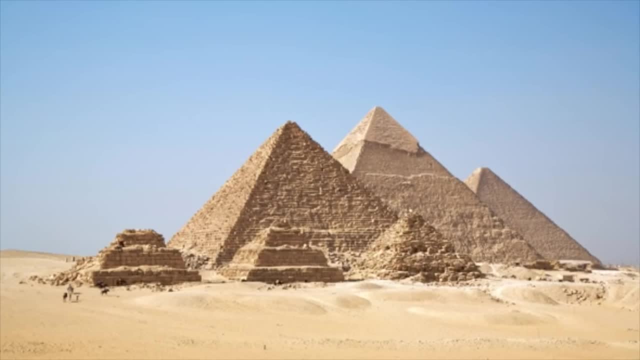 in separate pieces on a ship. But how did they get them on the ship? People couldn't have done it by themselves. They used mechanical advantage to carry the parts. There are many other examples of how mechanical advantage was used throughout history to move heavy objects such as the huge 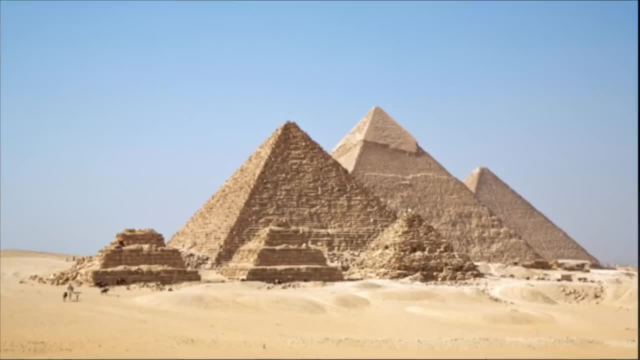 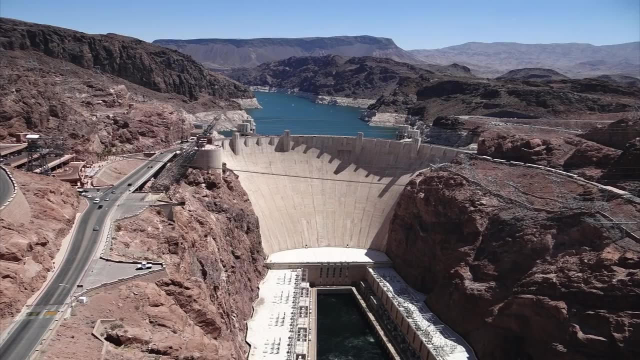 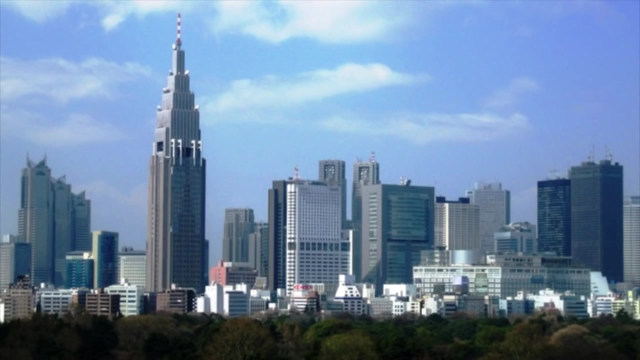 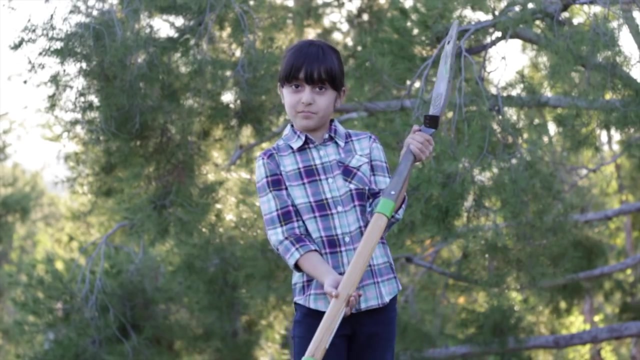 stuff: The stones making up the pyramids, the Stonehenge, the huge dams such as the Hoover Dam, and also the incredibly tall skyscrapers all over the world. One of the first devices used for mechanical advantage was actually the simple shovel. 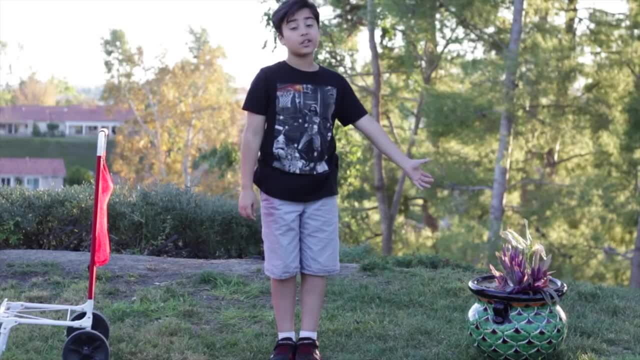 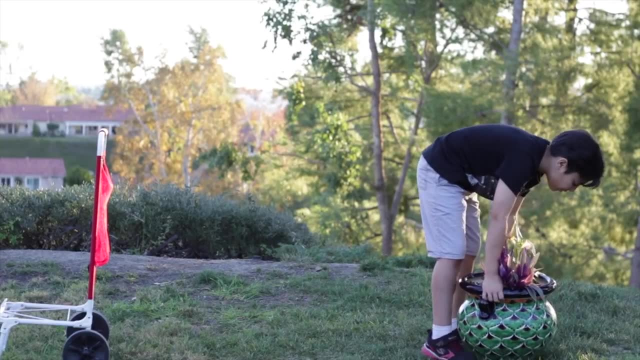 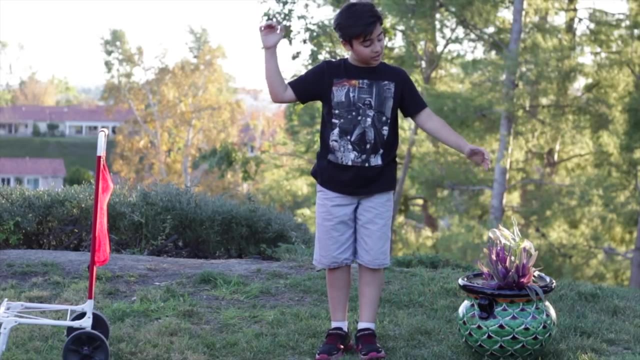 One example of mechanical advantage: Over here I have this extremely heavy pot which I am going to try to carry With this simple car. over here I am going to be able to carry this pot without any problems, which you shouldn't try this at home. So I am going to go ask my Dad for help, See if I can. easily do this. I have fun carrying my self made shovel and then move this to the program. Small by small, you can get this simple handle to spin. oh, journey, It's pretty hard, isn't it? But it can do this really easy. so feel free to add your creativity. Aàngam like using this tool, and